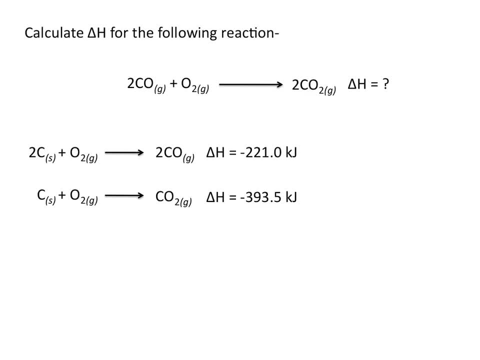 So we'll calculate delta H for this reaction, given the two reactions below and their delta H values. So the first step to do this is to manipulate the given equations so that they most closely resemble the equation of interest. So let's look at our first equation. 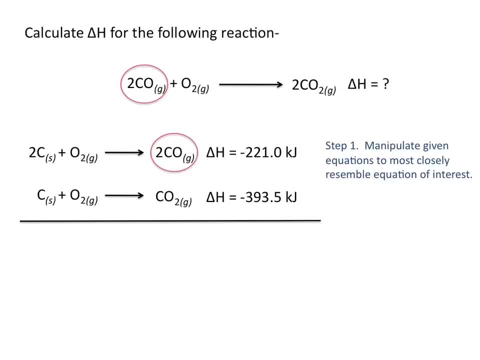 In the reaction of interest, carbon monoxide is on the reactant side, And of the two equations given below, you only see carbon monoxide in one of these equations, and it's on the product side. So what we're going to need to do is to flip this equation around so that 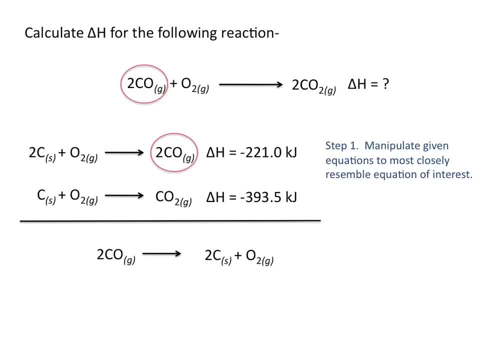 carbon monoxide is on the reactant side. So we'll write the equation below, except we'll flip it around. So here we have 2 carbon monoxide going to 2 carbon plus O2.. And because we flipped this reaction, we need to flip the sign on delta H. 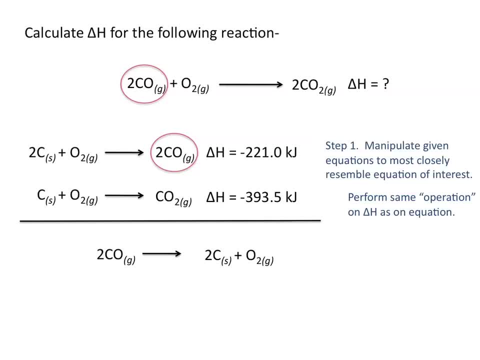 So remember, the delta H value for a reaction written in the opposite direction is of the same magnitude but of opposite sign. And so if we flip the equation, we flip the sign on delta H. So if 2 carbon plus O2 gives us 2 CO and the delta H value is negative, 221. 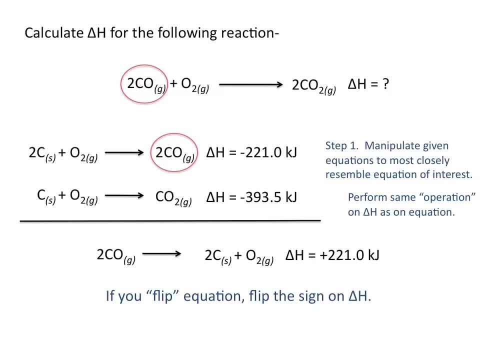 kilojoules per mole. then 2 CO going to 2 carbon plus O2 has a delta H value of positive 221 kilojoules per mole. Looking at our reaction of interest, I see that there are two moles of CO2 on the product side And when I look down at our given equations I see only one. 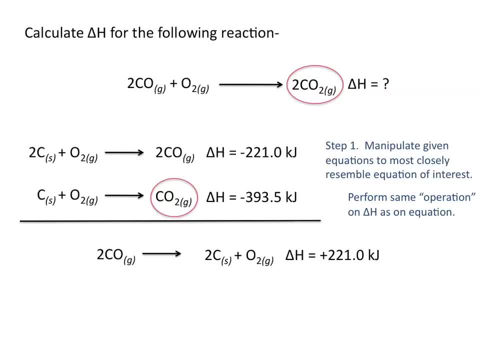 of the equations have CO2, the second one It is on the product side, but there's only one mole of CO2 in this reaction, And so for this equation I need to multiply it by two so that I have two moles of CO2, so it more closely resembles the reaction of interest. 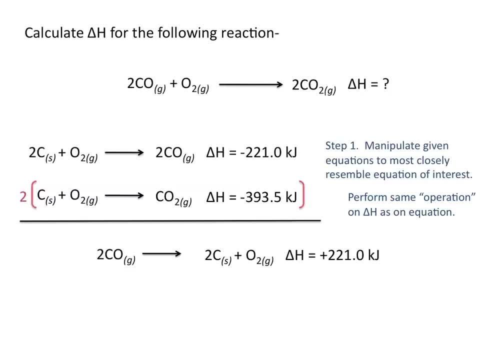 And when I multiply the reaction by two, I need to multiply the whole equation by two, And I think it helps to draw parentheses around the entire equation. So this gives us 2 carbon plus 2 O2, gives us 2 CO2.. And again, I want to perform the same operation in delta H as 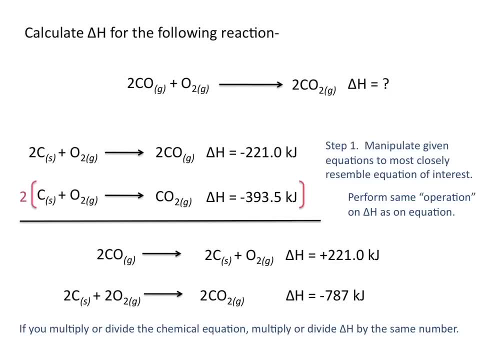 I did on the equation, And so if I multiply the reaction by two, the equation by 2, I need to multiply the Delta H value by 2. so if the reaction carbon plus o2 gives us co2, had a Delta H value of negative, 393, point 5. 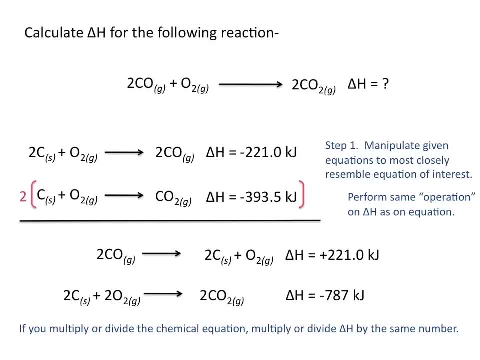 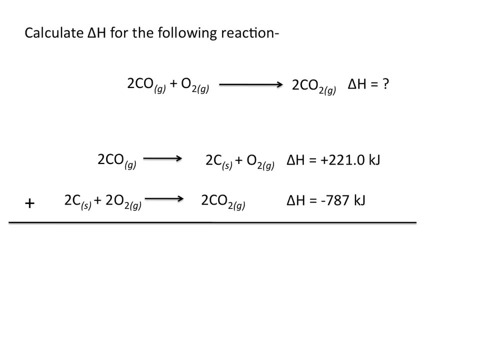 kilojoules per mole, then the reaction to carbon plus 202 gives us 2 co2 has a Delta H value of negative 787 kilojoules per mole. so here I've written my two new equations that I modified to more closely resemble my equation of interest. 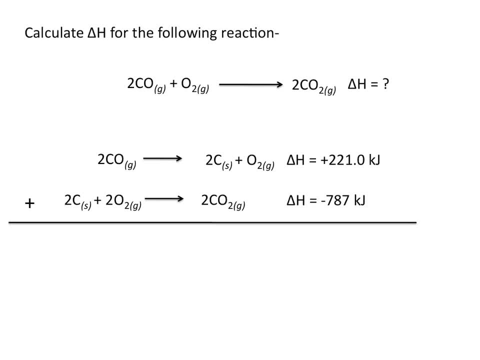 and what you're going to do now is add these two equations together, keeping everything on the reactant side, on the reactant side, and everything on the product side, on the product side. so in my new equation I have 2 co plus 2 C plus 2 o2, gives me 2 C plus o2 plus 2 co2. 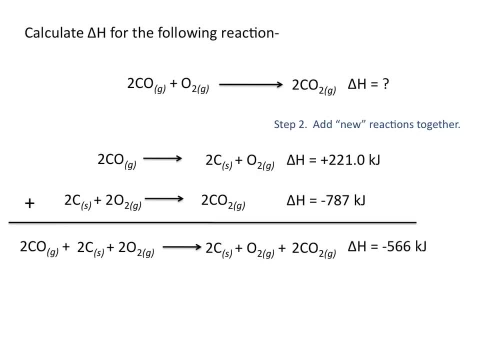 and because I added the reactions together, I'm going to add the Delta H values together. so the Delta h value for this equation is negative: 566 kilojoules per mole. but you'll notice that I have some compounds that are the same on both the reactants side. 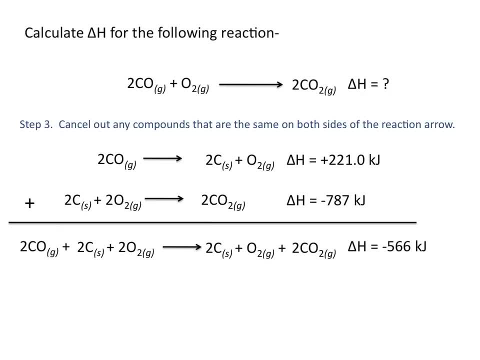 and the products side, and so anything that's the same on both sides of the reaction arrow can be cancelled out. so I can cancel out my two moles of carbon on both the reactants- the product side, and I can also cancel out the 1 mole of O2 on the product side. 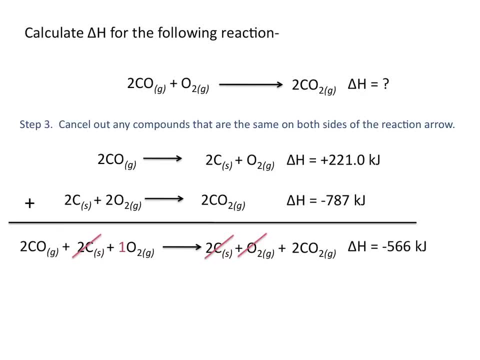 with 1 mole of O2 on the reactant side, leaving me with the final equation: 2 CO plus O2 goes to 2 CO2, and the last thing you need to do is to double check that this equation matches your equation of interest, and in this case it does so. the 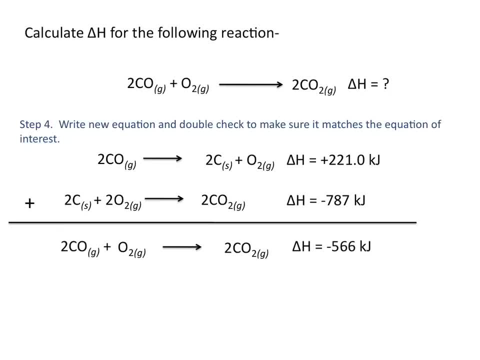 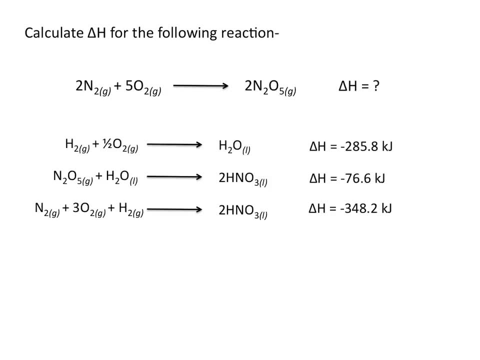 Delta H value for 2 CO plus O2 goes to 2 CO2 is negative 566 kilojoules per mole. let's try another example: calculate Delta H for the following reaction: 2 N2 plus 5 O2 goes to 2 N2O5. we're given three reactions listed below and 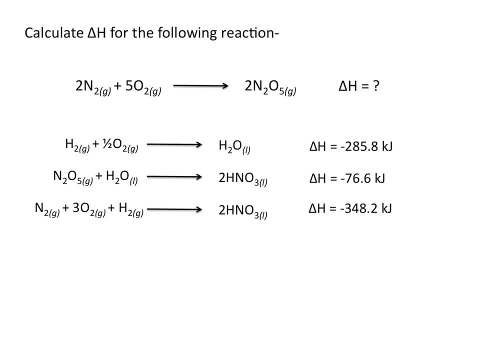 remember. the first step is to modify these equations to more closely resemble the equation of interest. now I think it's always helpful to look for a compound in the reaction of interest that is found only once in your given equations and in this case you can see the N2O5 that's on the product side in our reaction of interest is only one. 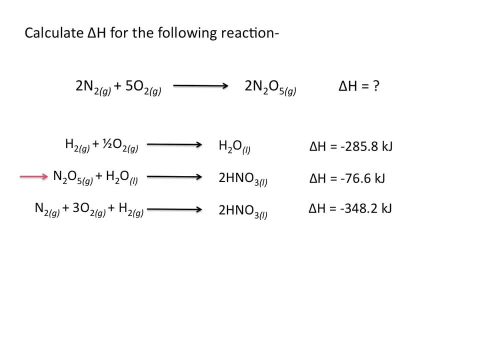 of the given equations and you'll see that it's on the reactant side. so the first thing we need to do is to flip this equation around so that N2O5 is on the product side. The other thing we need to do is to multiply this equation by 2, because 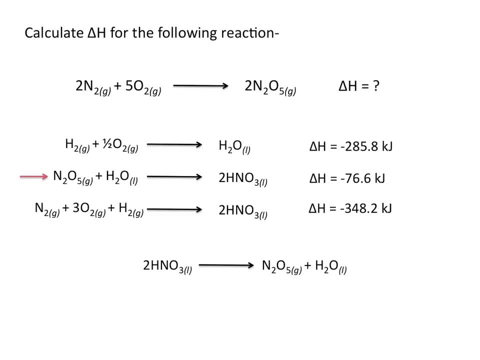 our reaction of interest has 2 moles of N2O5 on the product side. And remember, we performed the same operation on delta H as we did on the equation. So if we flipped the equation and multiplied it by 2, we need to flip the sign on delta H and multiply it by 2.. This 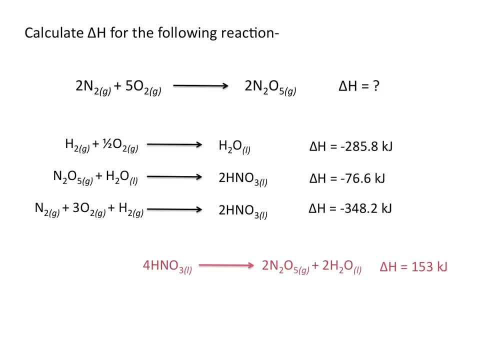 gives us the new reaction. 4HNO3 goes to 2N2O5 plus 2H2O and this reaction has a delta H value of 153 kJ per mole. Looking at the bottom equation, I'll see that I have N2 on the. 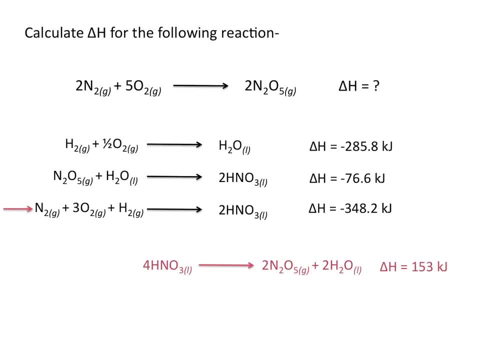 reactant side And in my reaction of interest I also have N2 on the reactant side. But in my reaction of interest I have 2 moles of N2 on the reactant side. So in order to make this equation, we need to multiply the reaction of interest by 2 and multiply it by 2.. So 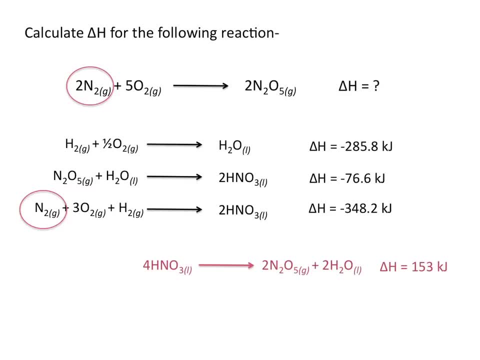 if this equation more closely resembles the reaction of interest, I need to multiply the entire equation by 2.. Now you'll also notice in this equation that 2 moles of HNO3 are formed on the product side, And when we compare that to the equation that we just modified, we 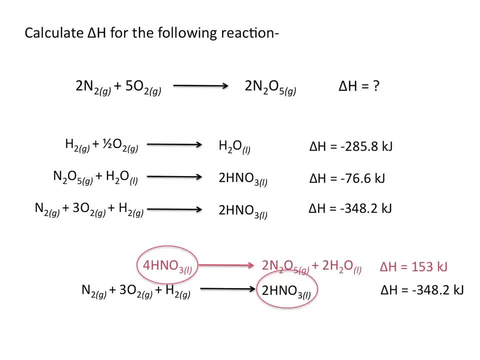 have 4 moles of HNO3 on the reactant side. If you look at our reaction of interest up on the top, you don't see the compound HNO3 anywhere in that equation, Which means that you're going to need equal amounts of HNO3 on the reactant side and the 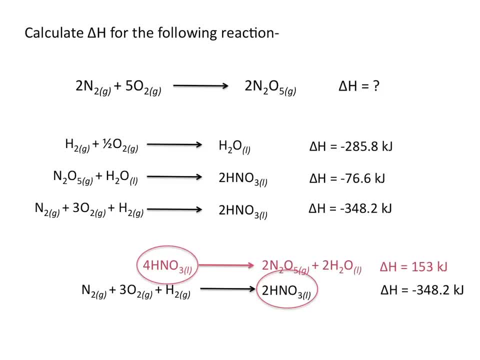 product side in order to cancel out in our final equation. So we already knew that we needed to multiply this equation by 2 to give us 2 moles of N2.. But you can also look at it that we need to multiply this equation by 2 to give us 4 moles of HNO3, which will 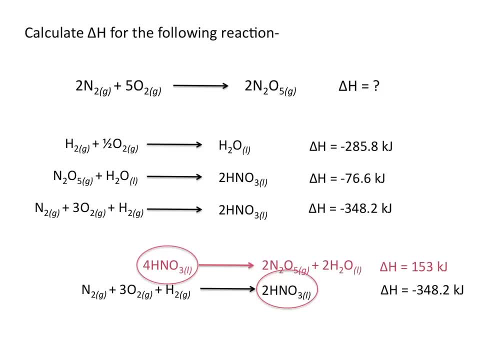 eventually cancel out with the 4 moles of HNO3 on the reactant side in our first equation that we modified. And when we multiply the equation by 2, we also need to multiply the delta H value by 2.. Now I saved this top equation for last, and it's because neither H2 nor H2O are anywhere. 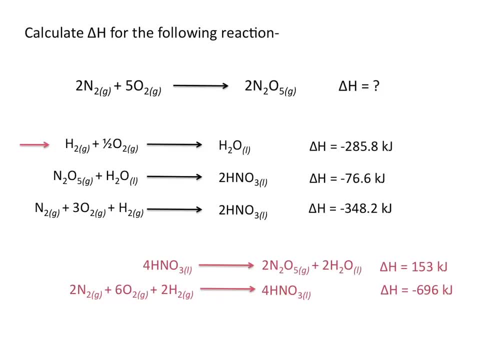 to be found in our equation of interest, And so we need to compare this reaction to the reactions that we already modified in order to figure out how to modify this equation in order to cancel out any moles of H2O or HNO3. 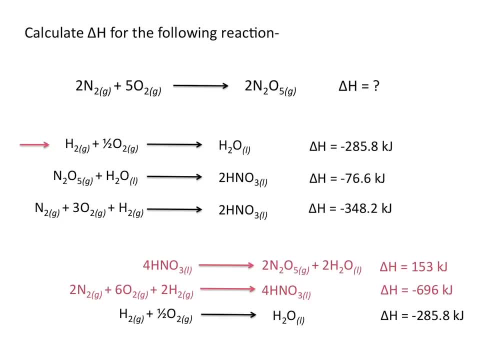 So here we have our H2O or H2 gas in our final equation And what you'll see is that we have 2 moles of H2O on the product side and we need to modify this third equation in order to cancel those out. So we'll need to flip this equation and multiply it by 2. 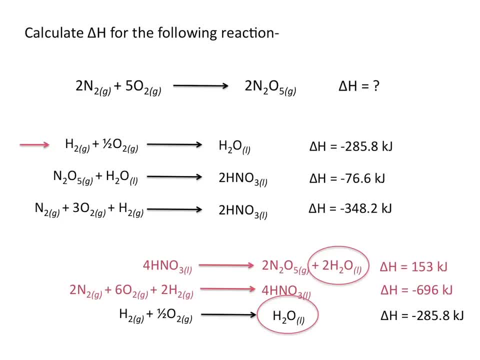 in order to cancel out H2O by having it on both the reactants and the product side, And you see the same thing with H2 gas. So when we flip this equation and multiply it by 2, remember that we need to do the same thing over and over again until we get the same. 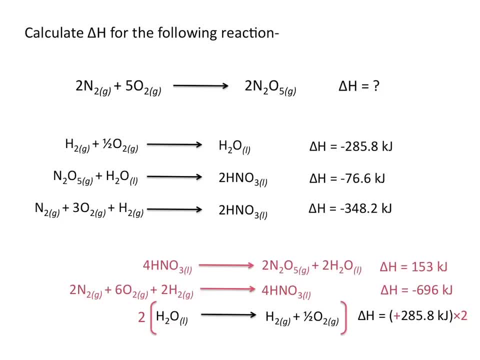 same thing for delta H. Flip the sign on delta H and multiply it by 2.. Now that we have 2 moles of water on the reactant side and the product side, those will cancel out when we add these equations together. And the same thing with our 2 moles of H2 on the reactant. 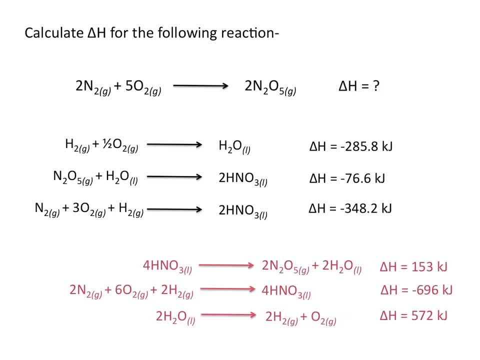 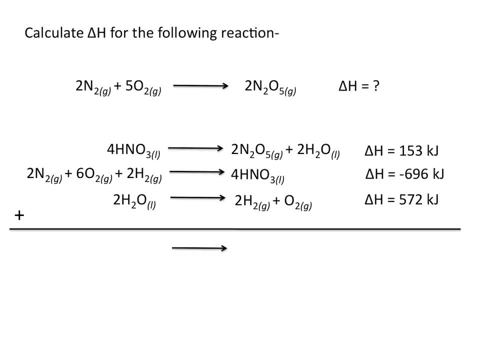 side and the product side. Now, hopefully we've modified all of our equations correctly, So remember, we add everything on the reactant side and everything on the product side, and then we can cancel out anything. that's the same on both sides. Now, if you don't want, 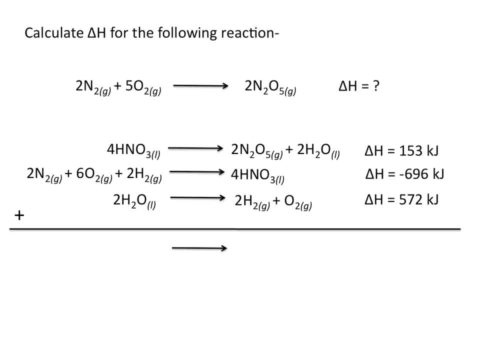 to write all of this out. you can cancel things that are the same on the reactant side and the product side right away before adding your equations together, And so you'll see that we have 4 moles of HNO3 on the reactant side and the product side We have 2 moles. 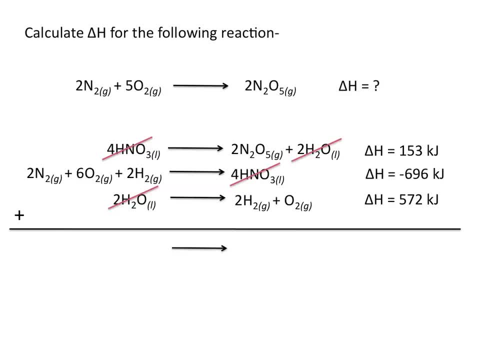 of H2O on the reactant side and the product side And we have 2 moles of H2 on the reactant side and the product side. Our 1 mole of O2 gas on the product side can cancel with 1 mole of O2 gas on the reactant. 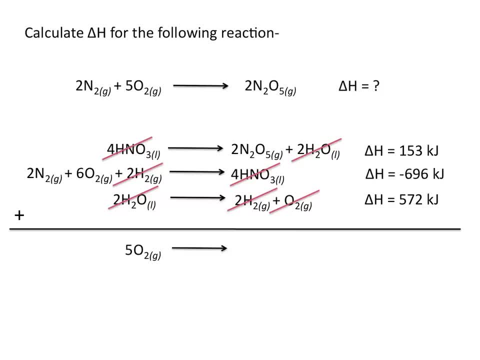 side, leaving us with 5 moles of O2 on the reactant side, And when we write down what we're left with, we then have an additional 2 moles of N2 on the reactant side and 2 moles 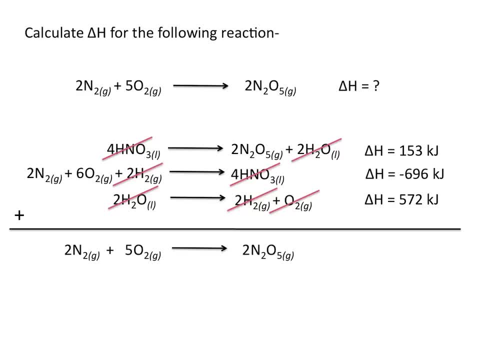 of N2O5 on the product side And when you check, our new equation now matches the equation of interest. And so, because we added up these 3 new equations, we now have 2 moles of HNO3 on the reactant. 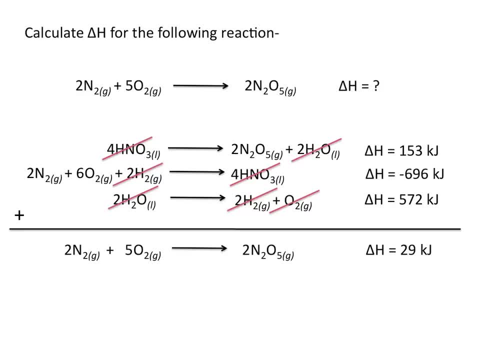 side, We also need to add up their delta H values, And so the delta H value for this reaction- 2N2 plus 5O2- goes to 2N2O5- is 29 kilojoules per mole. Thanks for watching The Chemistry Solution. We hope you enjoyed this tutorial. 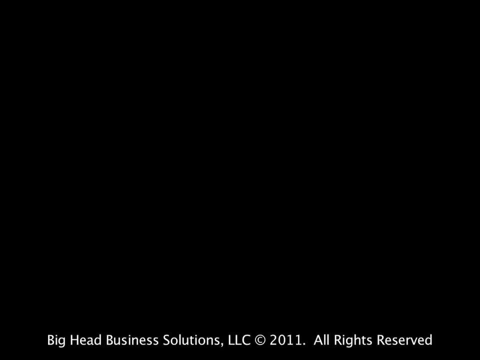 And we'll see you in the next video. 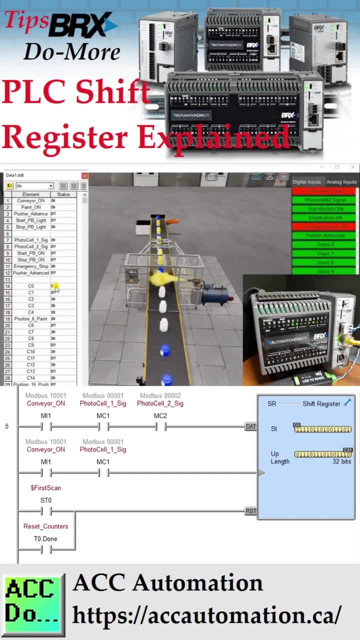 BRX DoMore PLC. Shift Register. The Shift Register SR instruction shifts bits through a predefined number of bit locations. These bit locations can be a range of bits, single words or double words, or a range of words or double words. This instruction has three inputs. 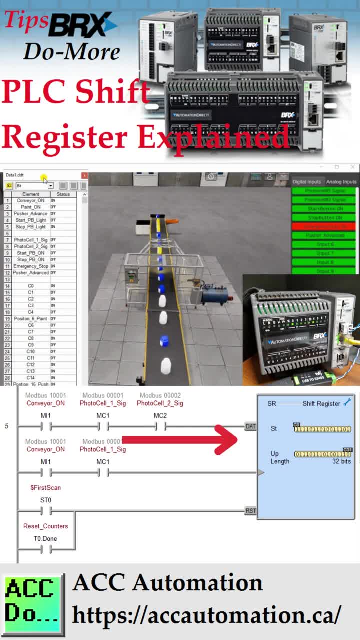 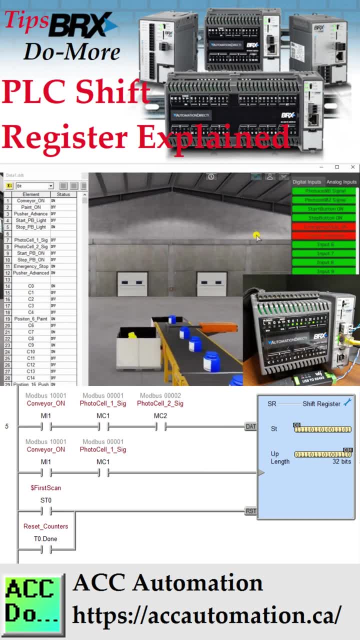 The first input is the data input. It will determine if a 1 or 0 will be placed in the first bit when the second clock bit input transitions from off to on. The third input is the reset, which will zero out all the bits in the Shift Register.